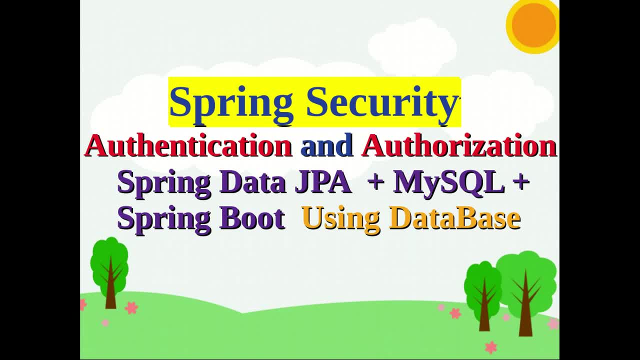 base and there we have hardcoded the username and the password in the application properties file. All right, and, guys, in this lecture we will get the credential from the database and we will try to validate that. All right, so let's start the development. So, guys, first of all, I am going 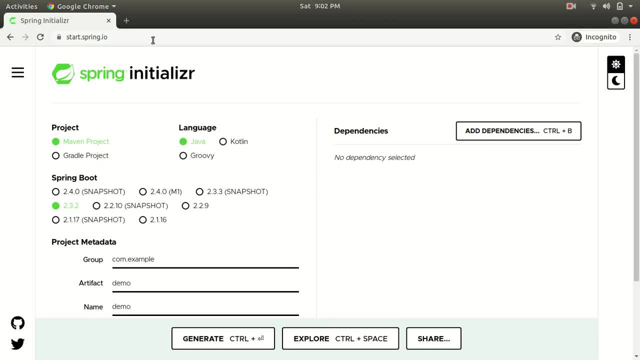 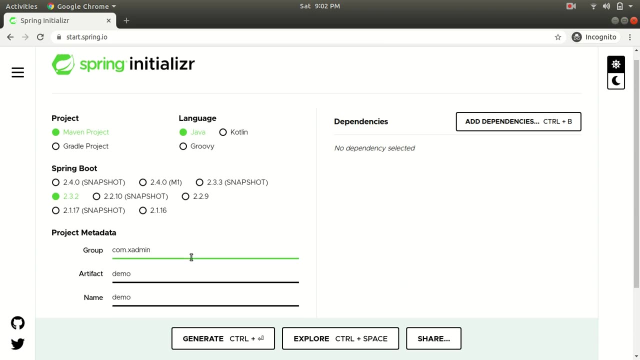 to create a Spring Boot application by taking the help of a Spring Inslicer, So this is by like a Maven project. Here is Spring Boot 2.3.2 I am using. So let's add a group here. All right, Let's. 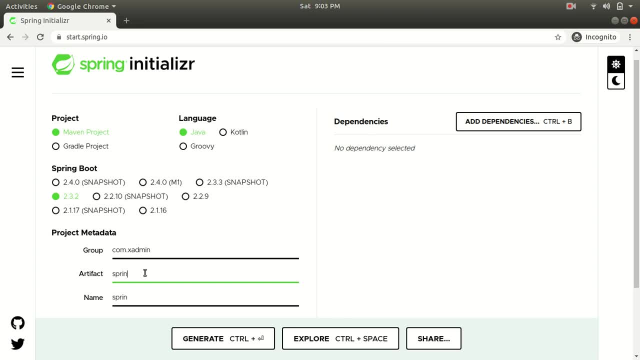 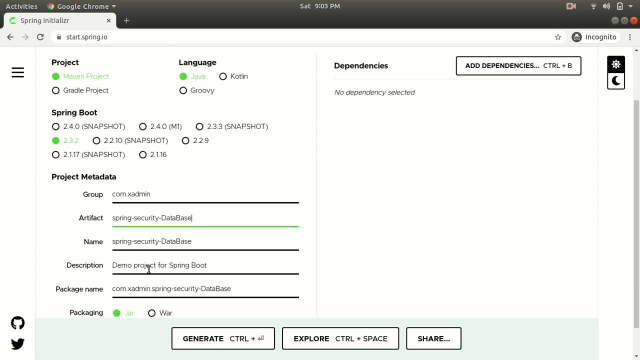 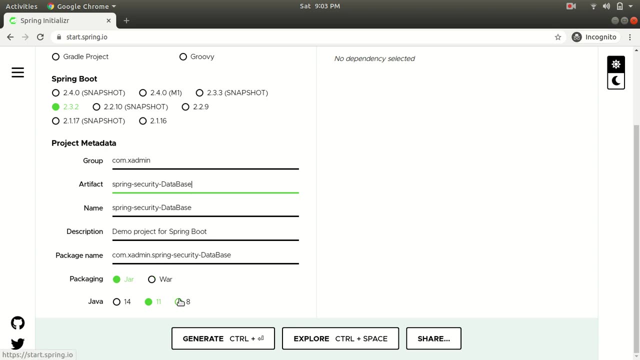 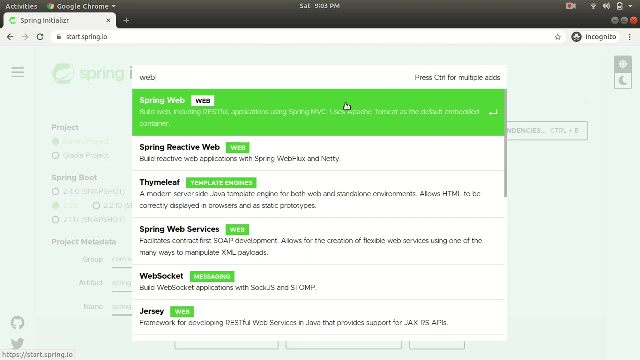 provide artifact name: Spring Security database. All right, Yeah, package name: in fine. So, guys, packaging I am going to keep as a jar and Java 8. to use. and now, guys, i will add the differences. so first of all, i will add spring wave. 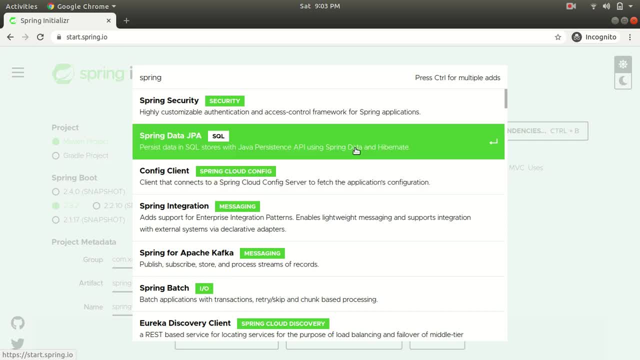 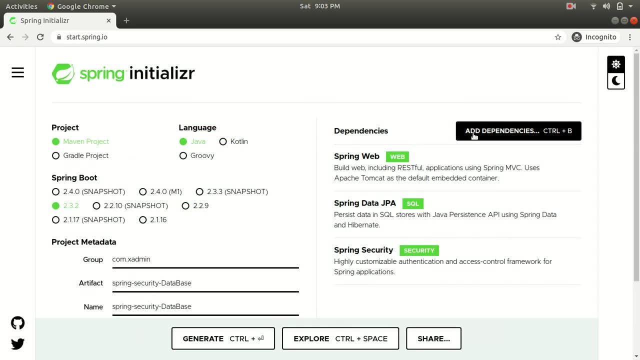 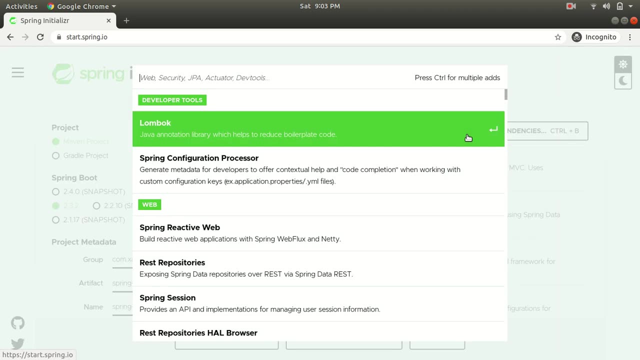 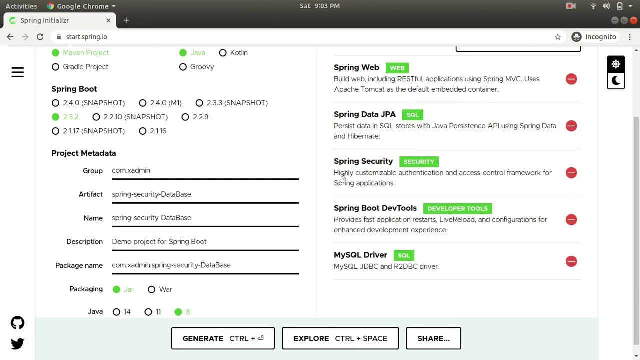 i will add spring data jpa, all right. i will add the spring security, all right. i will add dev tool, all right. and guys for the database, i will add, like the mysql driver. so guys, spring wave, spring data jpa, spring security and the spring data dev tool. 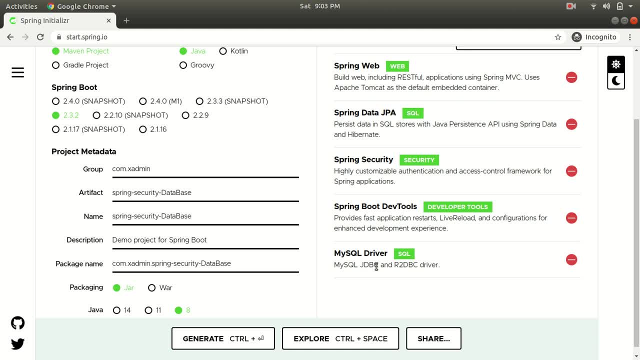 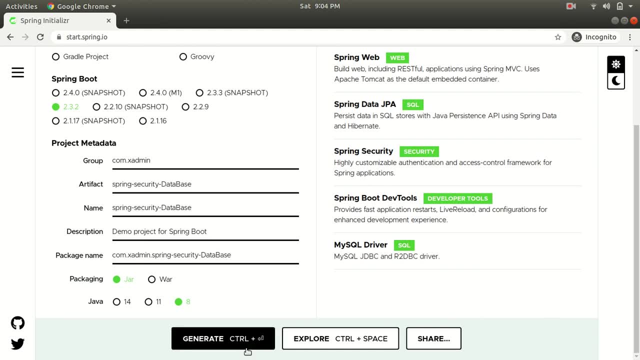 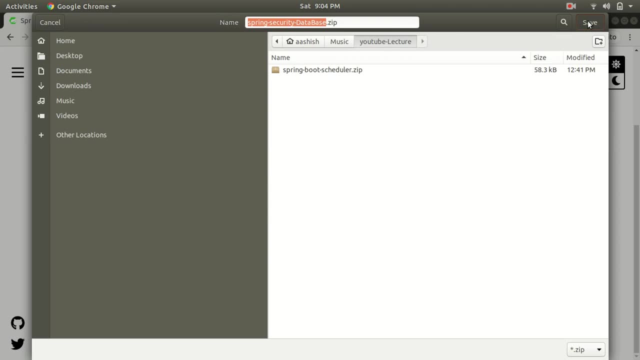 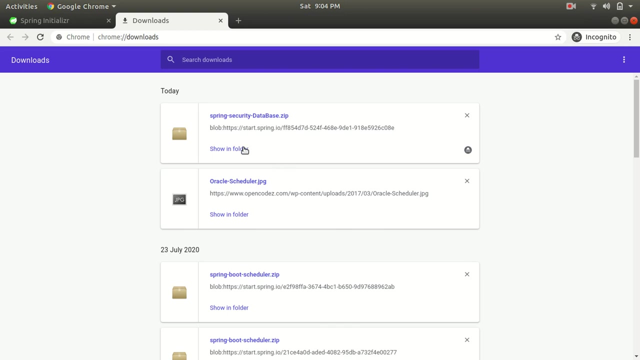 all right, and, guys, for the database i am using my sql driver. all right, so these are the dependencies i am adding to this project, so let's generate our project. so, guys, our project will be downloaded in a g format, so we need to extract it. and then we need to import to our eclipse. so we have downloaded, so let's extract it. 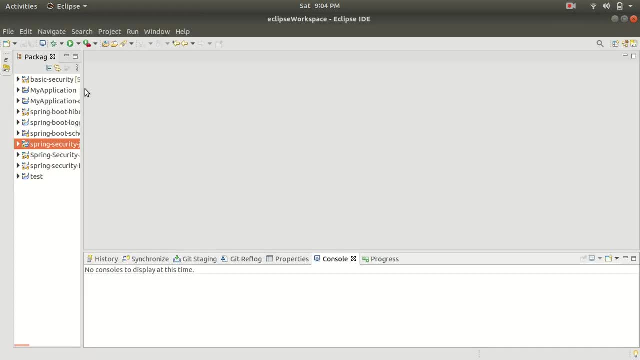 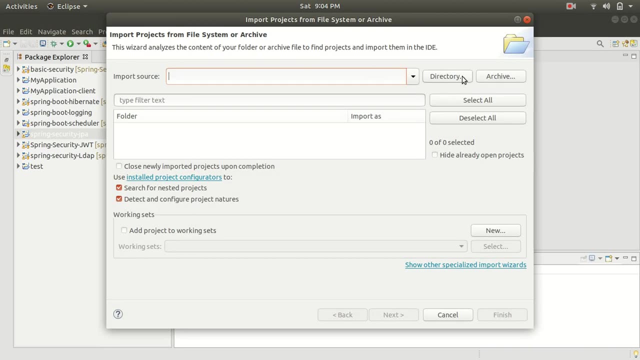 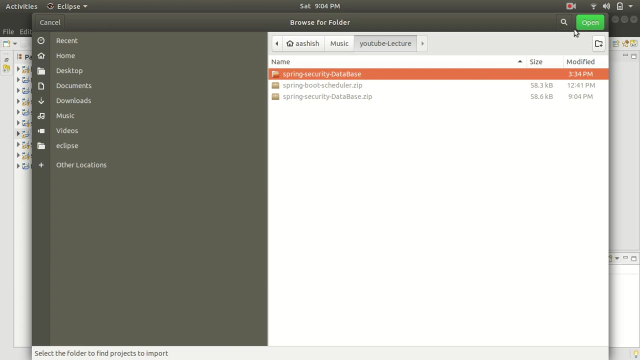 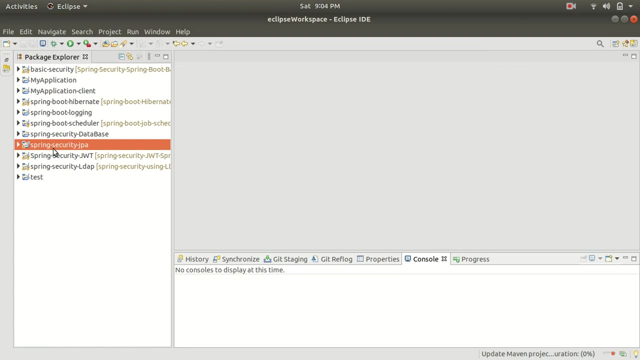 let's go to our eclipse, and here we need to import the project, so provide the path directory. all right, so this is my project, so just open it and finish it. guys, we have successfully imported this spring security database in our eclipse, all right, so now, guys. so, guys, you can see that we are updating, and all right, so project is updated. 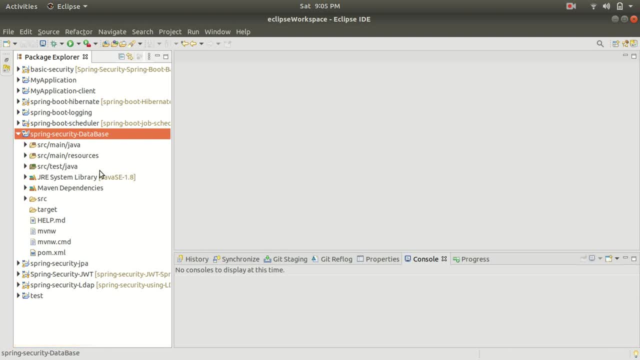 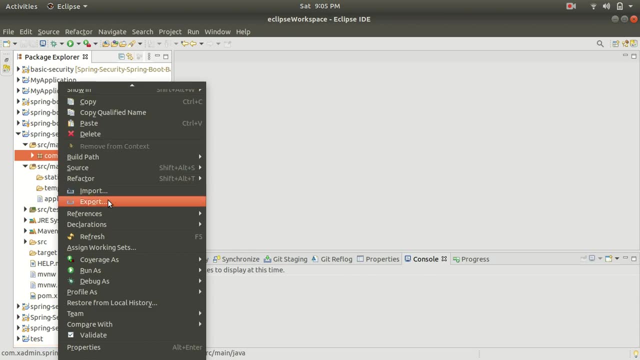 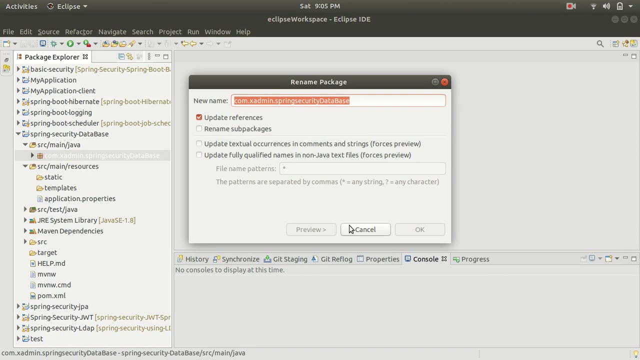 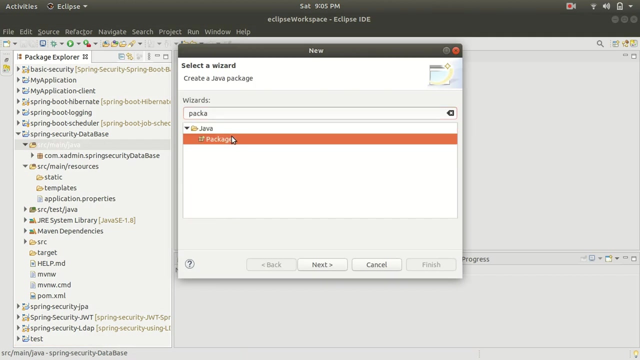 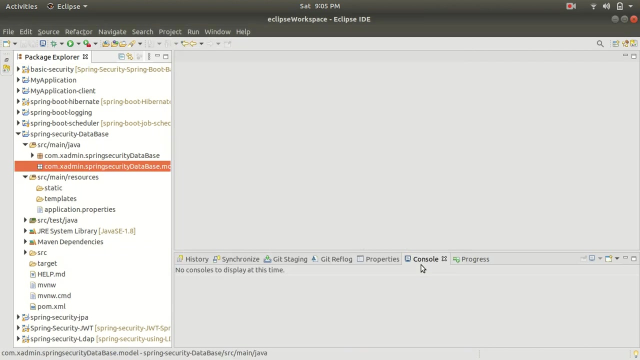 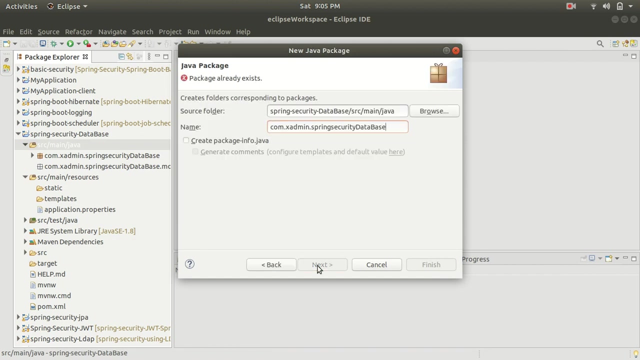 all right, and now, guys, i am going to create all the packages which we are going to use. so let me copy this package. let's create a package. so, guys, the first package. i will create a model package. so, guys, inside the model package, we will create model classes. all right, so next package, i will add, as a controller: 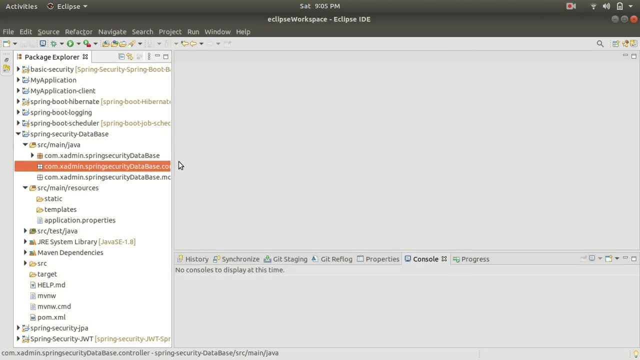 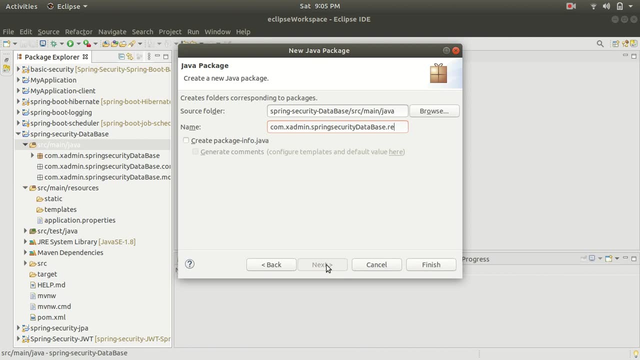 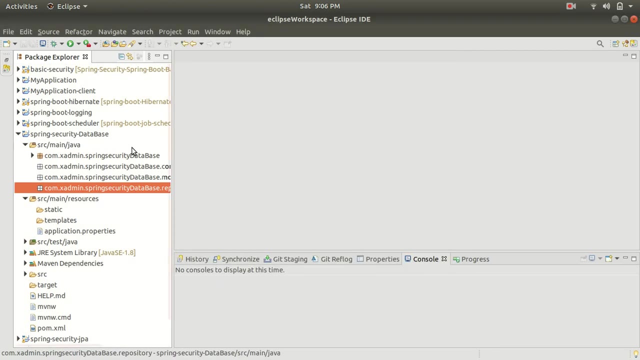 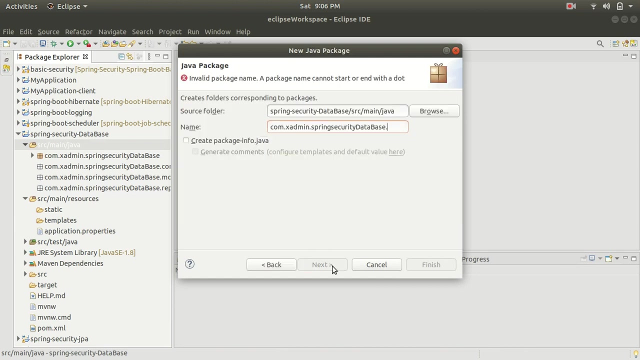 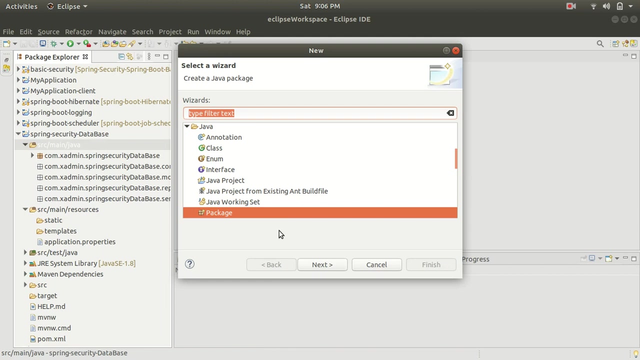 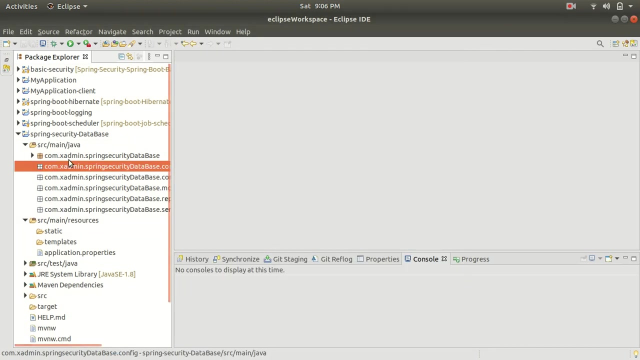 in which guys we will add controller class. next package: i will add the repository repository- finish this. next package: i will add service package- finish, so next package. so next package i am going to add as a config package. all right, so these are the packages i have added to my project, all right? and 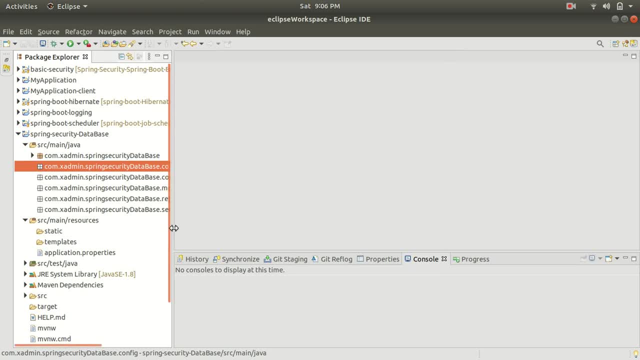 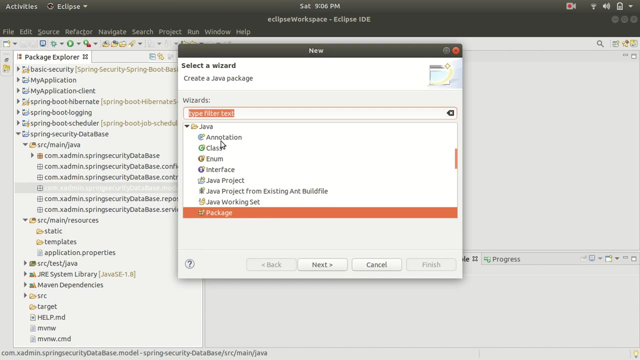 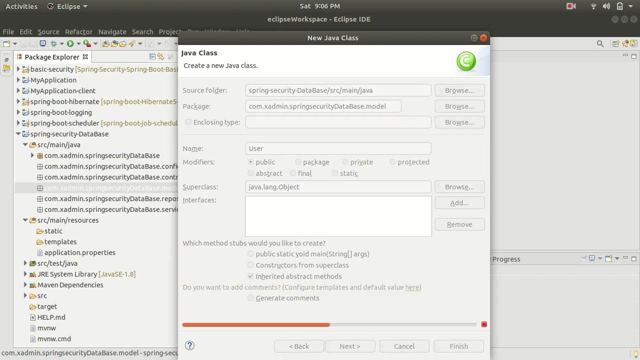 now, guys, i am going to create the model class. so, guys, i am going to create the user class and, guys, the user will contain the information like user id, username, password and the email. all right, so inside the model class model package, let's create a class with the name user. finish this. so this is our user class. so mark this class as an entity class. 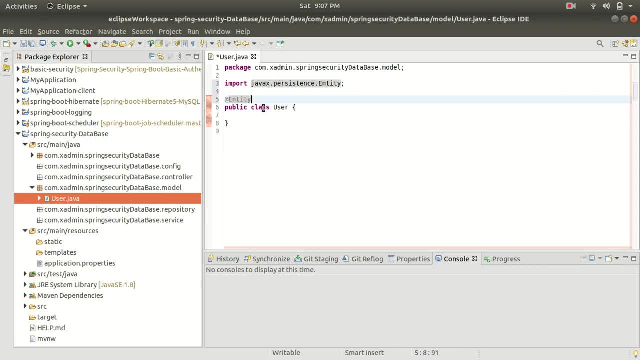 to make this as an entity, all right. so, guys, it will create the table with the name user inside our mysql database. so, guys, here the user class has the following properties, like: private end user id: all right. it has a username of a string. return type, data type: all right. 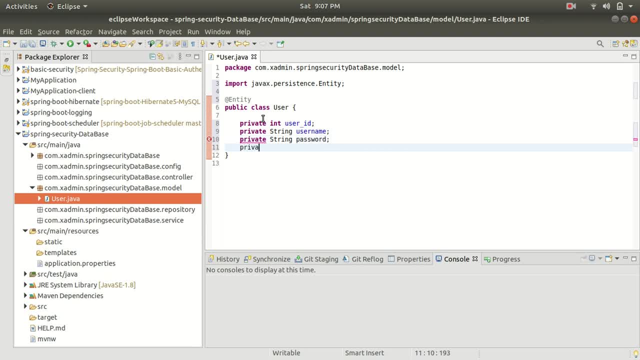 it has a password. it has an email. so these are the information we have added to our user model: class, user id, username, password and email. all right, so, guys, here i want that user id should be auto generated, and, and, guys, it should be a primary key. so let me mark this with the id annotation for the primary key, and let me mark this. 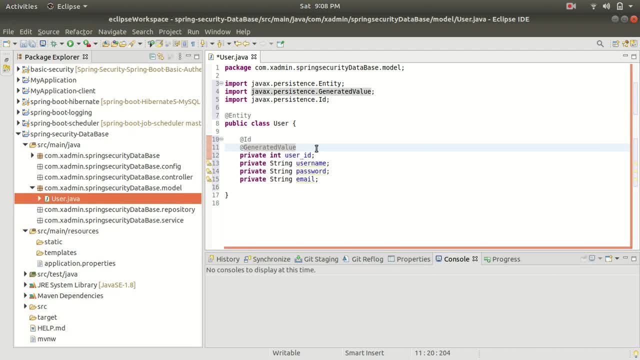 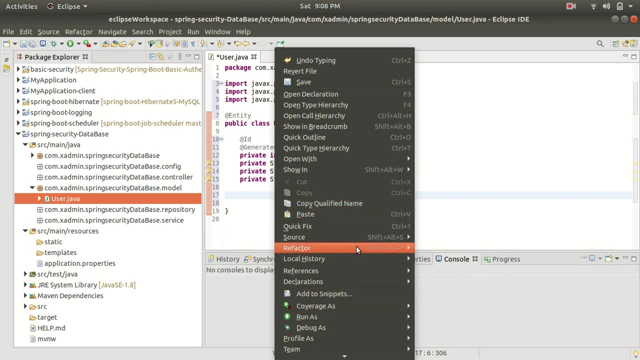 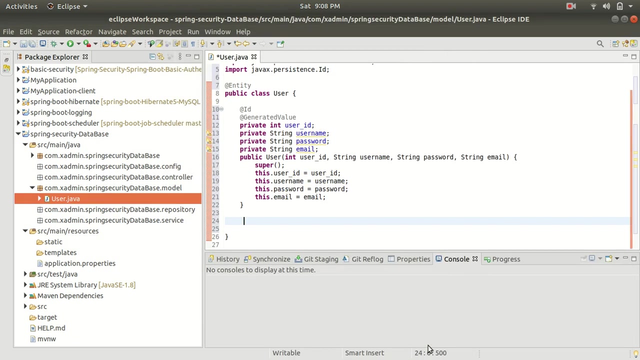 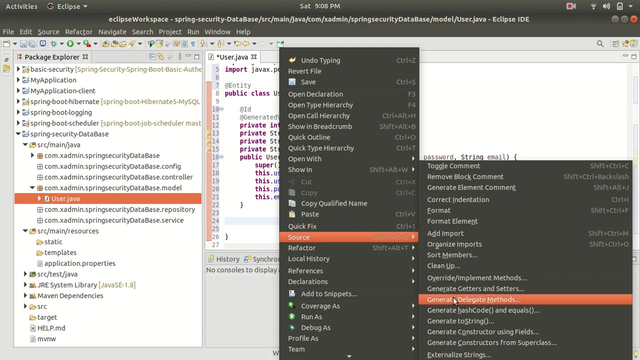 with the generated value to generate the id automatically. all right, so now, guys, i am going to. so now, guys, i am going to create the constructor. so let's generate the constructor, select all, generate, and here i will generate a default constructor also, and now i have added what we've named here, ah, and select all. 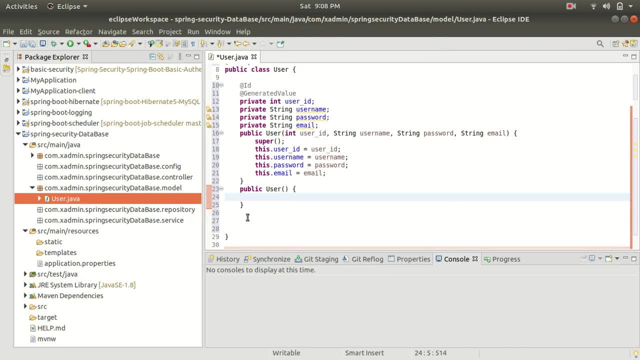 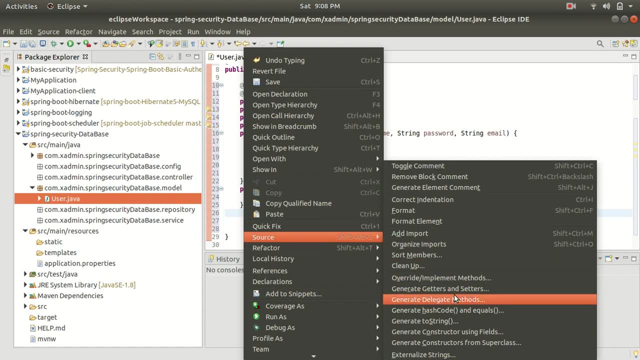 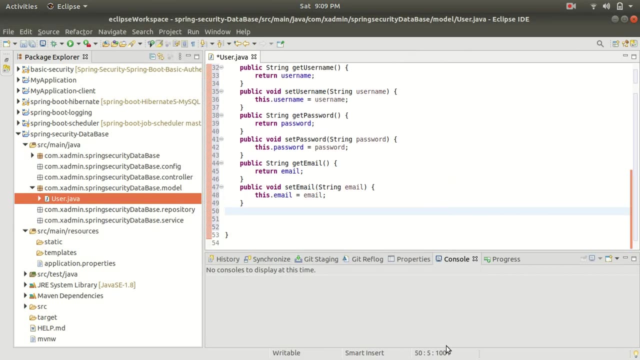 generate. all right, i put the default constructor now so I need not to turn off the keyboard. but okay, so now it's okay. so now i have come to the configuration and I can set it all. i can put all the Saturn method from here. all right, do i can set? 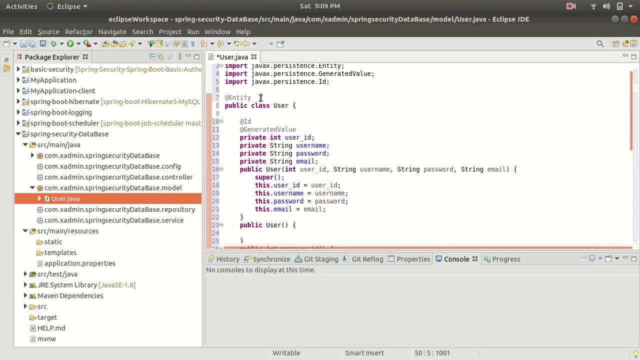 and put all the Saturn method from here also can review all amount for every user. okay, so now, if I have added this as entity class, so that it is going to create a table with the name user inside our mysql database and user id is a primary key and also it is auto generated, 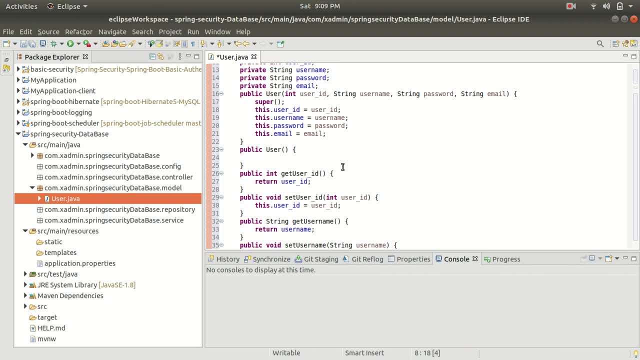 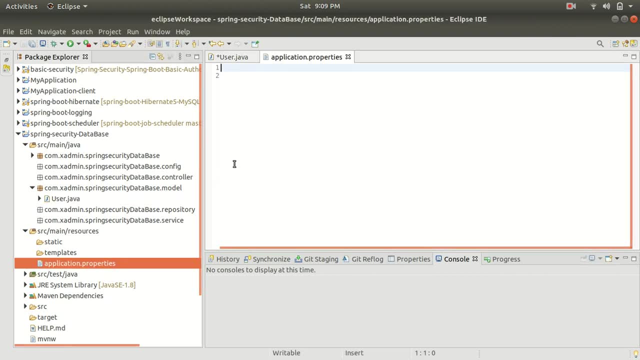 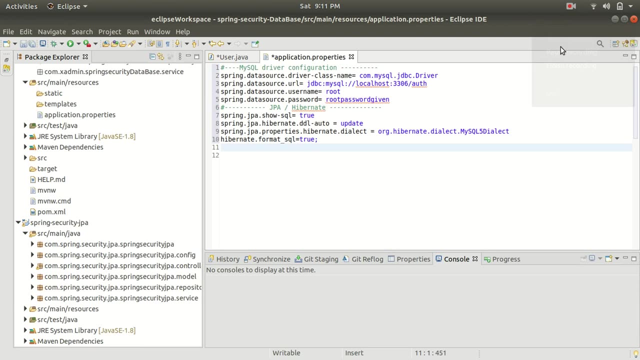 all right, and now, guys, i am going to add the configurations inside our applicationproperties file and the configurations like the mysql database configuration. all right, so guys, so guys, let me write the configuration and then i will explain you. all right, guys, i have added the configurations like mysql driver configurations, and here you 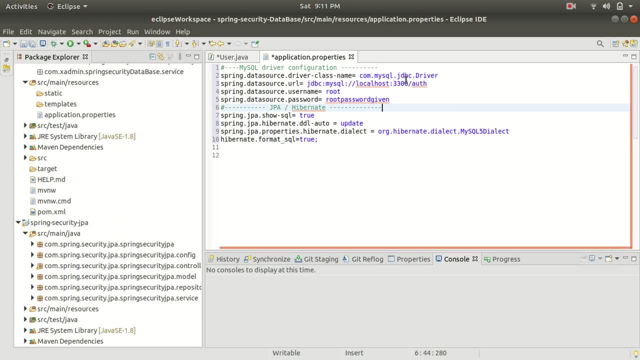 can see that spring data source driver class name is commysql- jdbc driver and we have the url like jdbc- mysql, localhost and guys. here i am using the default port, that is 3306, and my database name is auth. all right, and we have the username as root and the and guys. this is my password and. 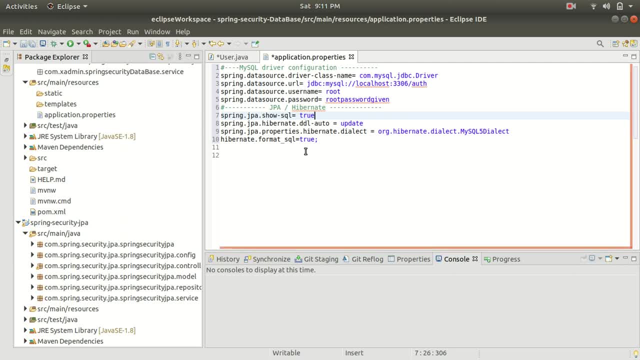 guys, here i am adding some hivernate configurations, like i want that to show the sql so true and the ddl auto is update, all right. and, guys, here i am using hivernate dialect as mysql 5 dialect and the format sql is true. so these are the configurations i have added to. 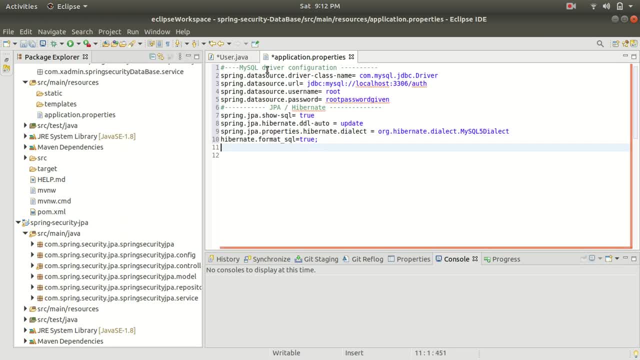 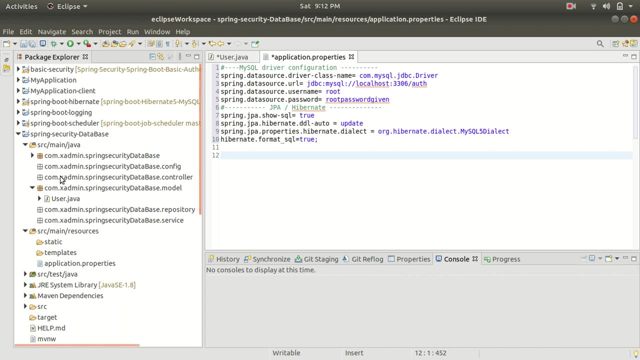 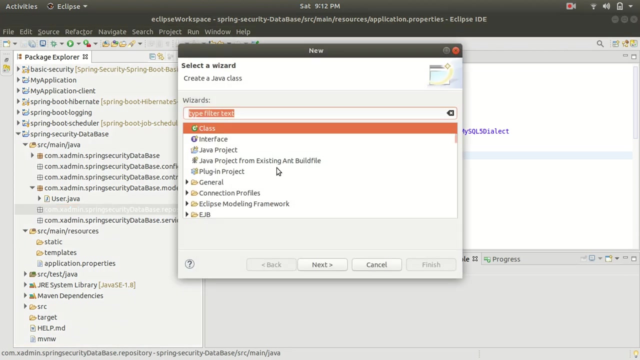 my applicationproperties file, and this is related to the mysql driver configuration and also the configuration related to the hivernate. all right, so now, guys, i am going to create the user repository. so let's go to our. now, guys, let's go to our here, the repository folder, and here i will create one more class. 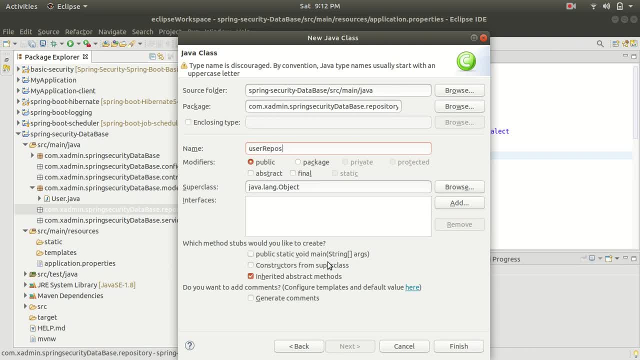 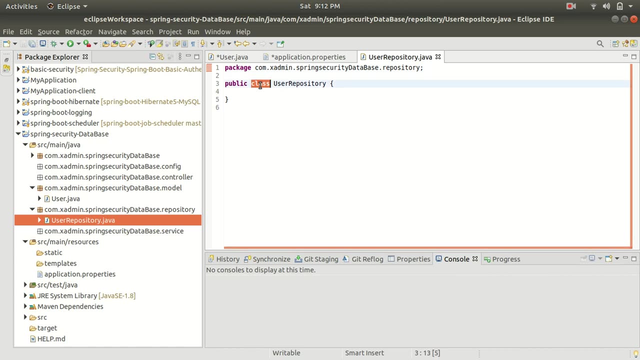 with the name user repo z3. all right, so finish this. so, guys, this is my the user repository. so, guys, it should be a interface. so change it. all right, user repository is interface and i will extend this interface with the jpa repository, all right. so here, guys, we have to pass our entity class, let's say user. 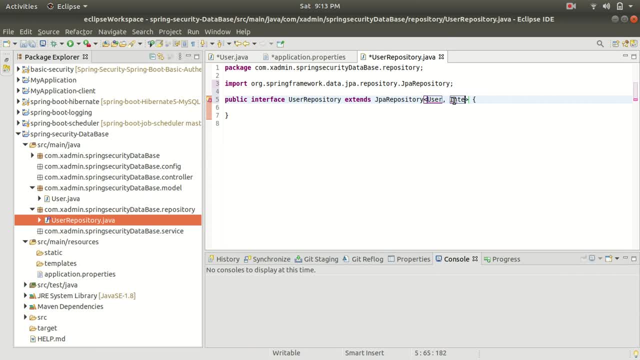 and our id. the primary data type is like integer. all right, so we have to import user with the correct package, model package, all right, so this is our like a repository interface in which we- i am extending with a jpa repository. so, guys, all all the current operations will be handled by 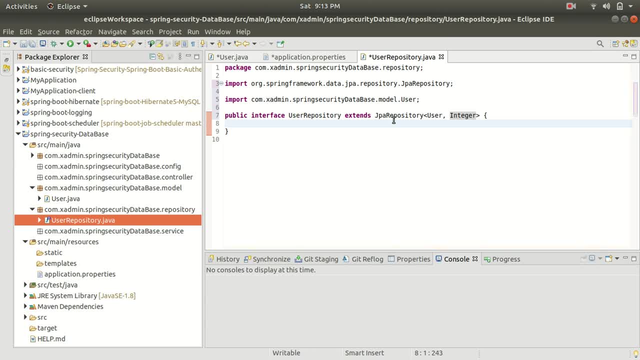 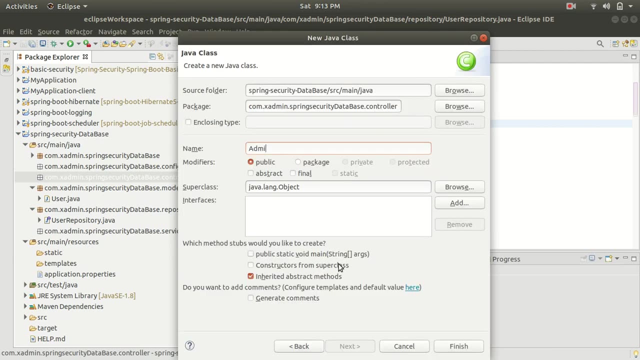 this, okay, jpa repository. so now, guys, i am going to create a controller for the rest endpoints. so let's go to the controller package and here create a class. so let's create a admin controller with the name admin controller. and, guys, inside this controller i am going to write a endpoint. 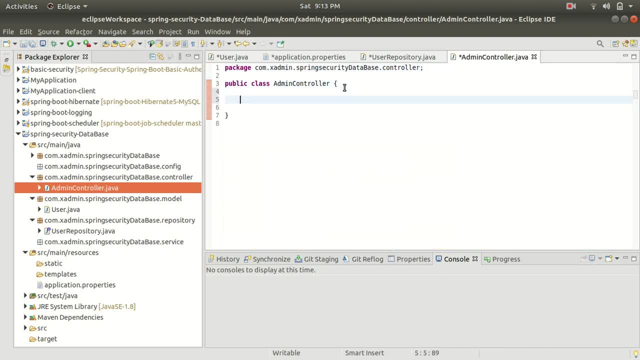 which is going to add, add the like, add the user data in the database. all right, and, guys, here i will not use any spring security to add any user data to the database. we will directly add the user data to the database. so, guys, first of all, i will mark this with the rest controller. 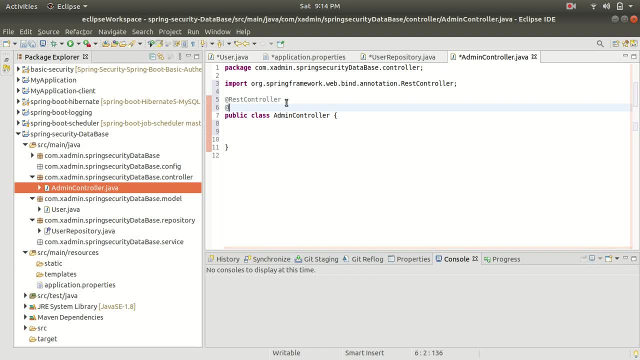 all right. so let's provide a request mapping and let's provide the url, so i will keep url as secure, or just, yeah, secure both. all right. and now, guys, i am going to, and now, guys, i am going to create the endpoint to add the user object to the database. so let's create a method: add user by. 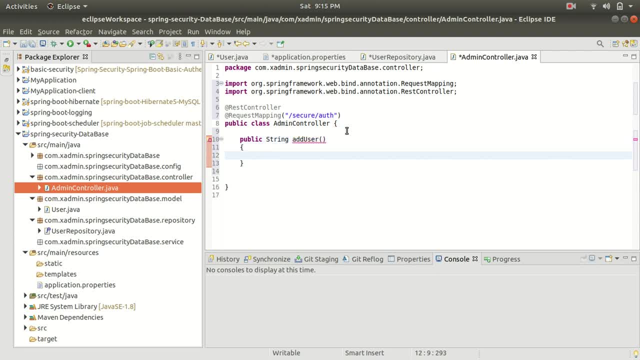 all right, add user. so here, guys, i am going. so, guys, here we have to take the user object from the request, from the request body. so for that, guys, let's say user. so import with the correct model class and here we will use at the rate request body to get to get the user object from. 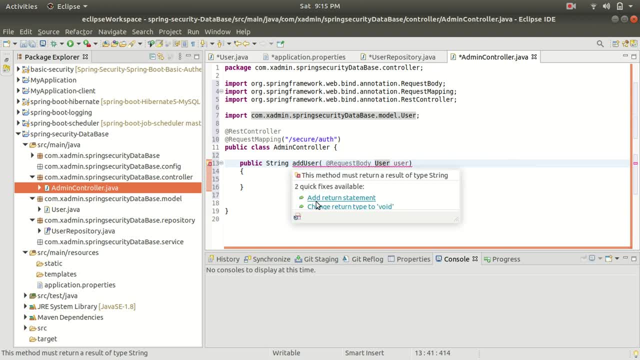 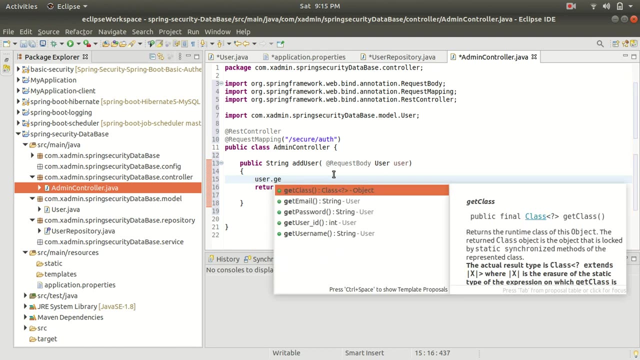 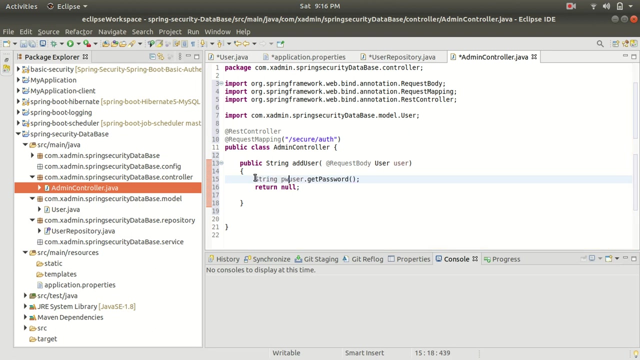 the request header, all right, so let's add a written statement. and now, guys, i am going to, and now, guys, i am going to take the password from the request object, all right. so user dot get password. all right, and i will store this in a string. so, guys, i took a password from the request header, object: all right, and i have stored in a. 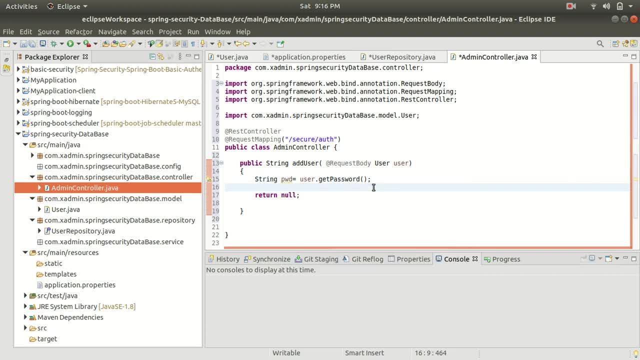 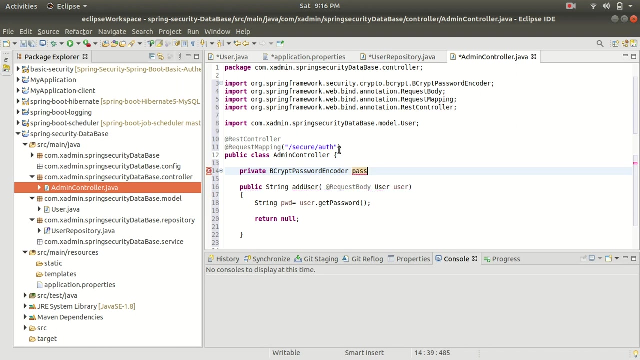 pwd variable string. and now, guys, what i will do. let's string encrypted. so now, guys, i am going to call a password encoder, all right? so first of all, i have to inject the like the password encoder. so private, private password encoder. so let's now name this as a password encoder, all right? so, guys, with this password encoder, 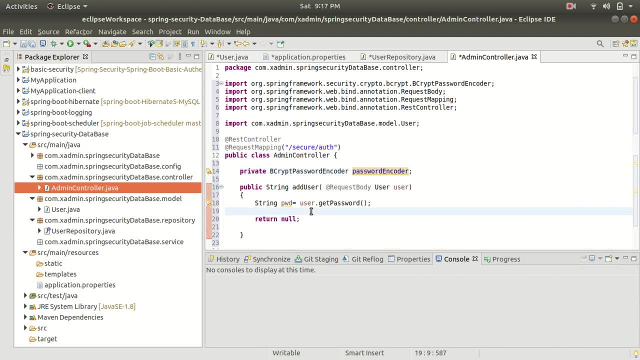 all right, with this password encoder, i am going to call the encode method and here i am going to pass our pwd variable, in which we have stored the password from the request header. all right, so let's store this in a encrypted pwd variable variable. all right, and now, guys, i am going to set the password to the user. so, guy, so, 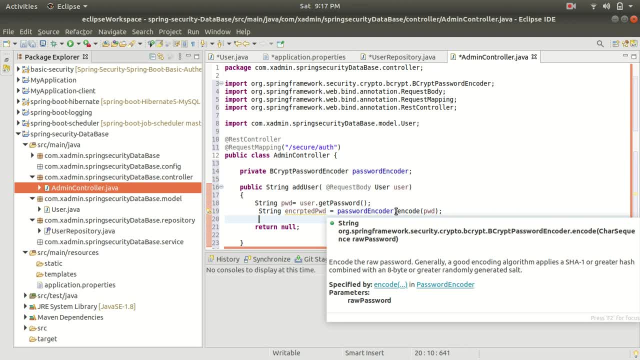 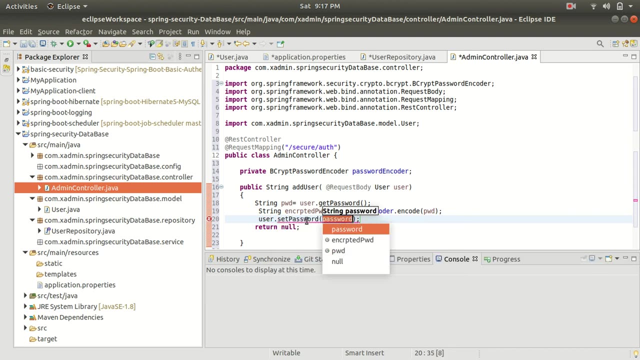 guys here. guys, it is going to encode the password. all right, and guys and guys here, it is going to encode the password. so now we need to set the password to the user object. so let's use the user object to set the password, let's call set password and here we can pass encrypted. 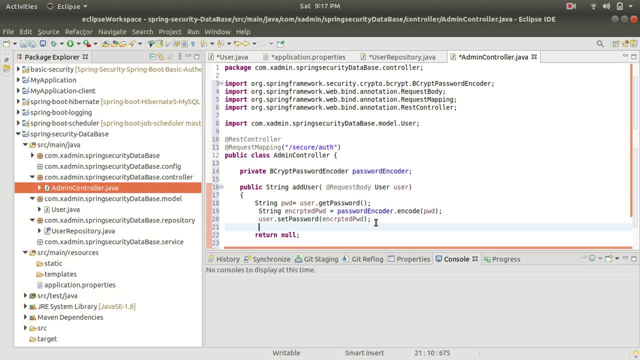 pwd. all right. so, guys, here we are taking the password from the request body and then we are encoding that password. and now, guys, we return this password in a encrypted form, in encrypted form string, and then we are setting in: it means we are saving this password to the password. 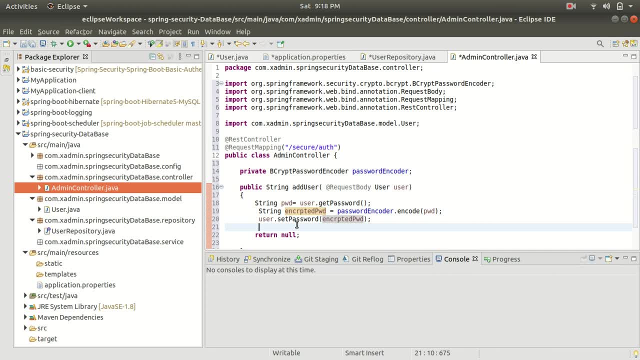 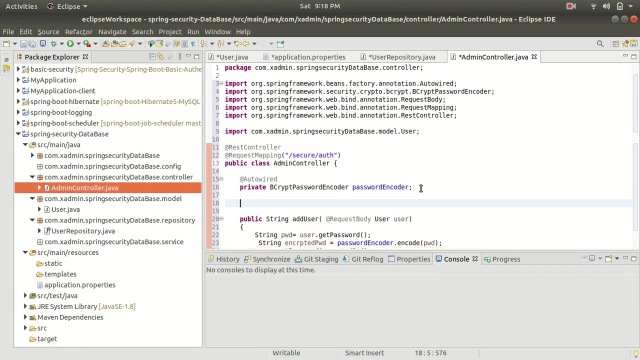 key of the user model, all right. and now, guys, we will call the save method of the user repository. so, guys, let me add this auto wire. and now, guys, i need to inject the user repository here. so let user repository, all right. user repository to our wire, all right. 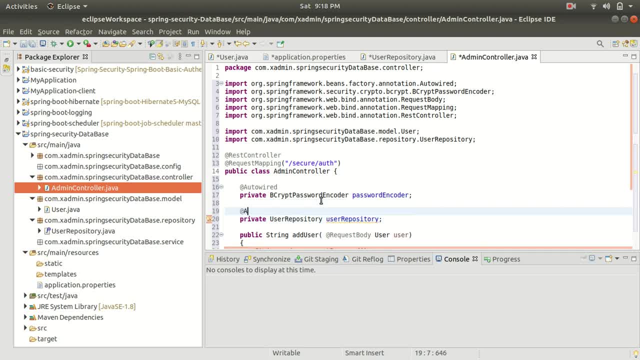 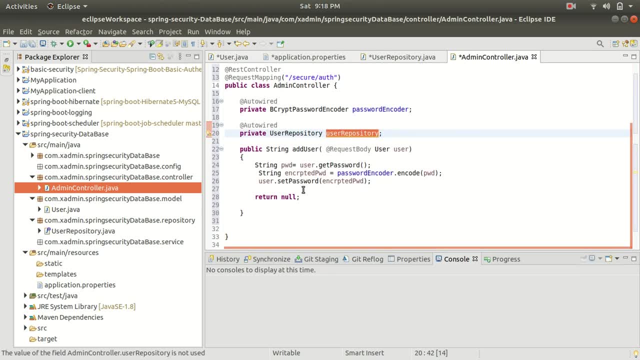 so let's annotate that, this with the auto wire. so, guys, i will call the save method with this user repository. so save, and here i will pass my user object. so, guys, it will save the user to my mysql database. all right, and here i will return a dummy string after adding the data to the. 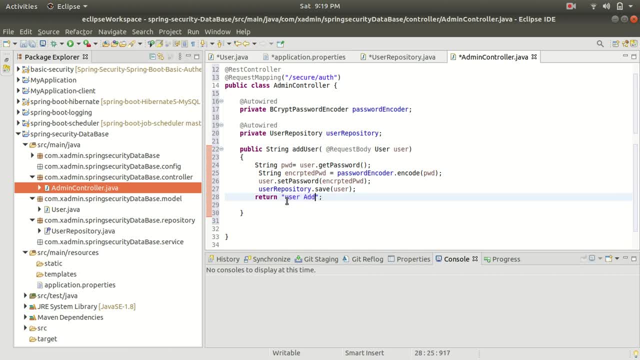 database. so user added successfully, all right. so, guys, i have passed a dummy string, so let me mark this with the post mapping and let's provide some url like admin and add. all right. so, guys, i have created an end point to add a user data to the database. all right, and now, guys, i am going to 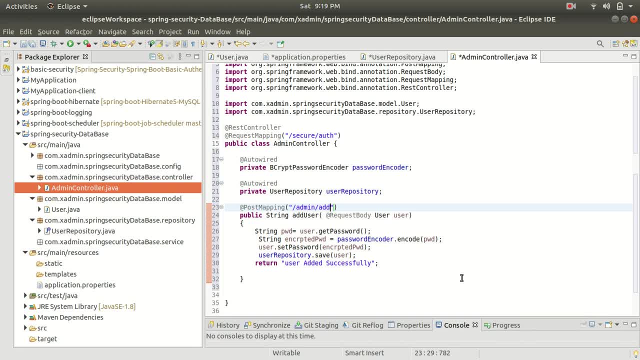 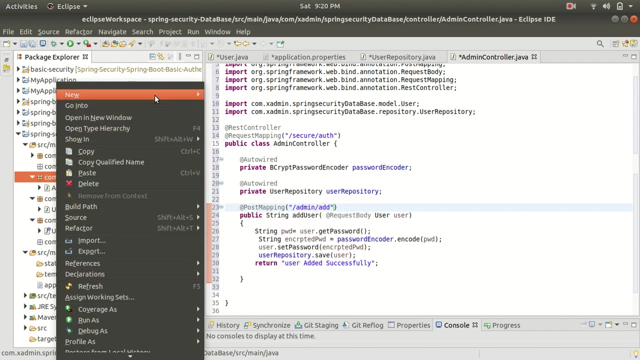 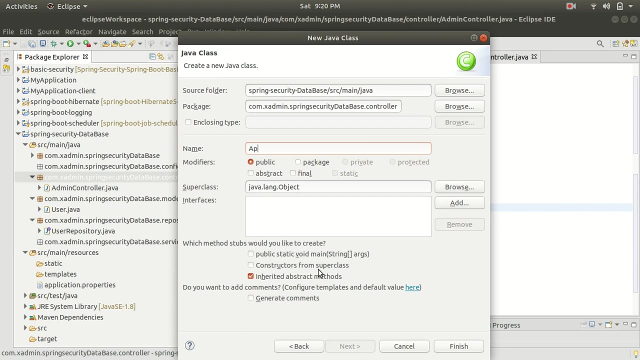 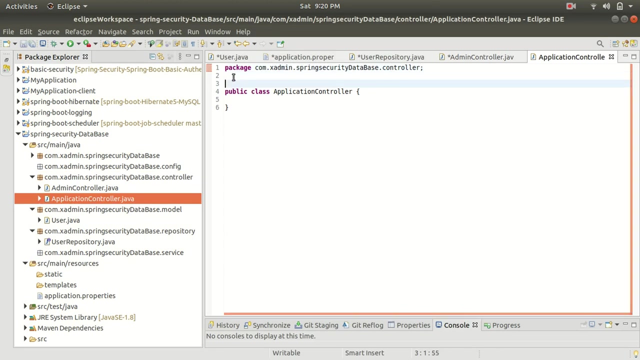